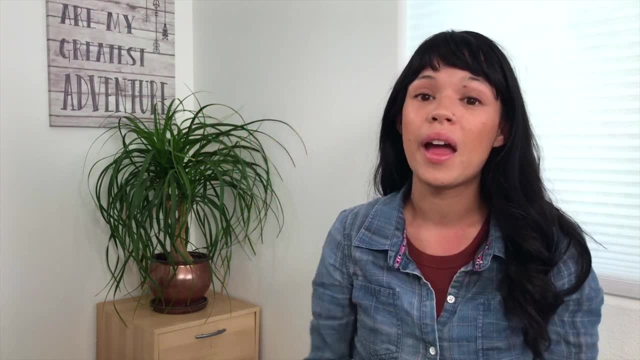 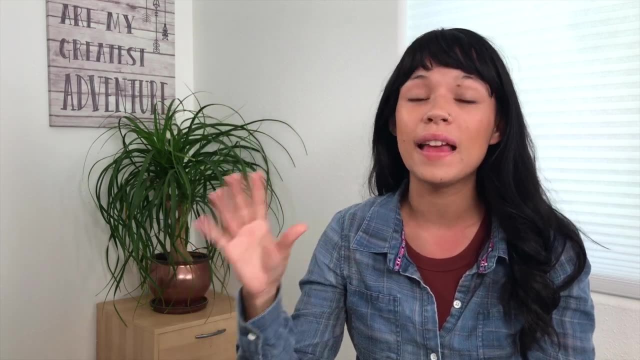 do need to be taught that do fall under this language arts umbrella. Just to kind of break the fourth wall here a bit, I'm actually going to look over here because I have a list of just some of the concepts that I was able to find just by Googling. what do kids need to? 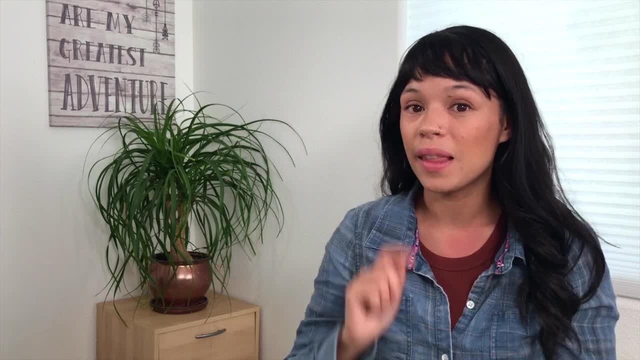 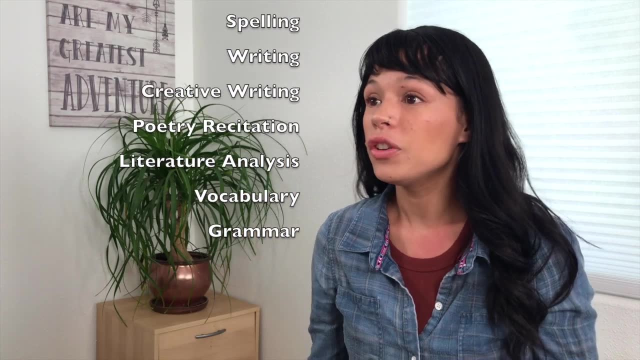 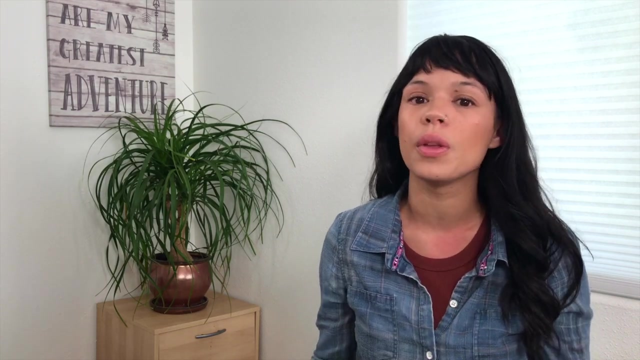 learn in English or language arts. So let me read this list to you now: Phonics, reading, comprehension, spelling, writing, creative writing, poetry, recitation, literature, analysis, vocabulary, grammar. This is a lot, and this isn't even all of the ones I found. I just started typing the. 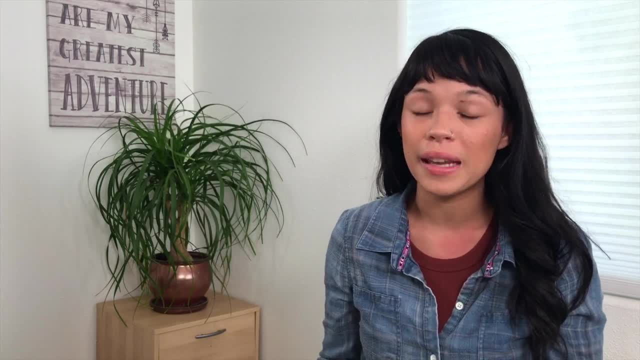 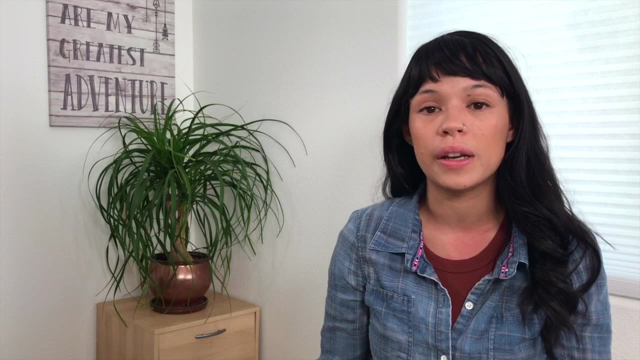 first few that I found. So I know this can be overwhelming and that's why I say: just stick to one at a time. A really good example for this is Stacy's oldest son is now in third grade, so he will be participating in our state standardized testing. So she has really been 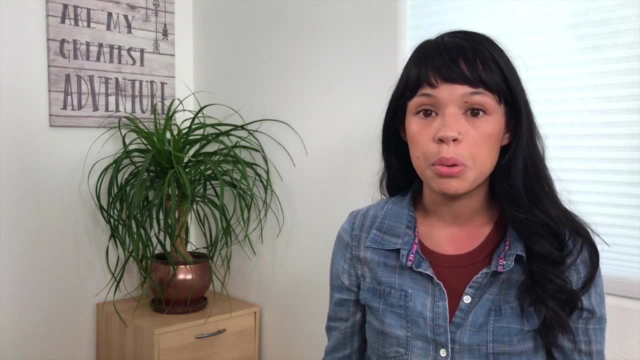 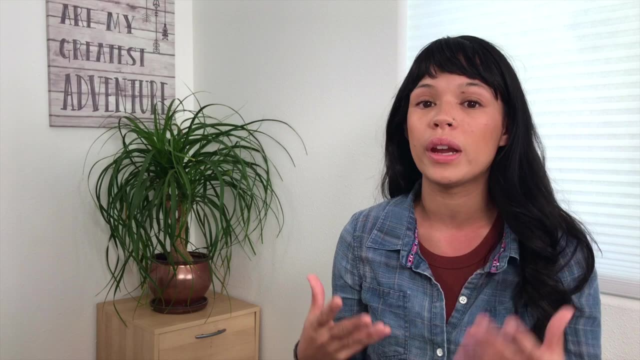 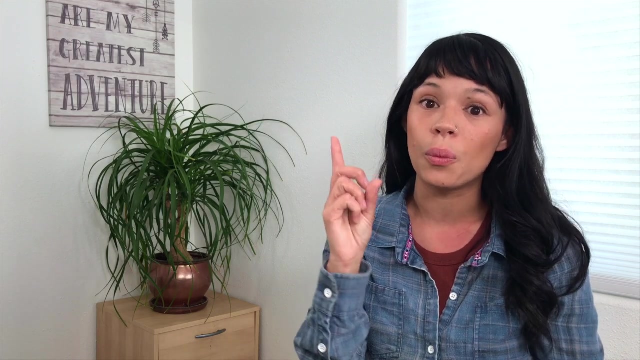 focusing on him succeeding in that writing portion of the test. So she has been really just focusing on writing for him. So writing paragraphs, maybe even doing some creative writing sentence structure, all of that It's actually easier said than done, but once you give yourself the freedom to just focus on one concept at a time, 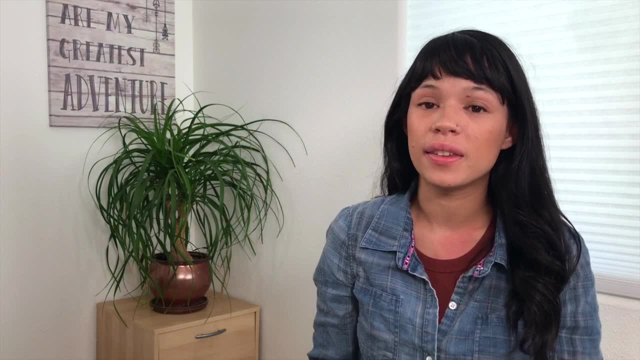 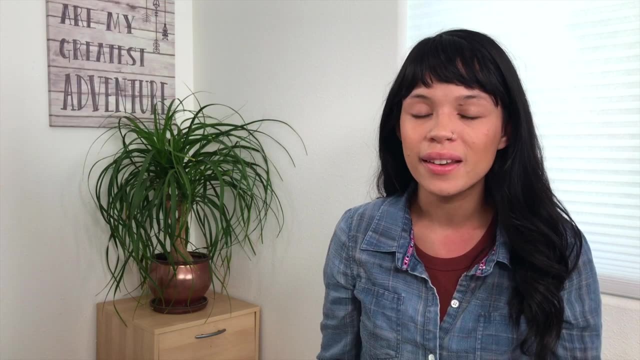 you will be good to go. Another thing I do want to add to this concept of focusing on one concept at a time is that exposing your kids to good books and having them read a lot will actually naturally expose them to concepts like grammar and sentence structure and creative writing. 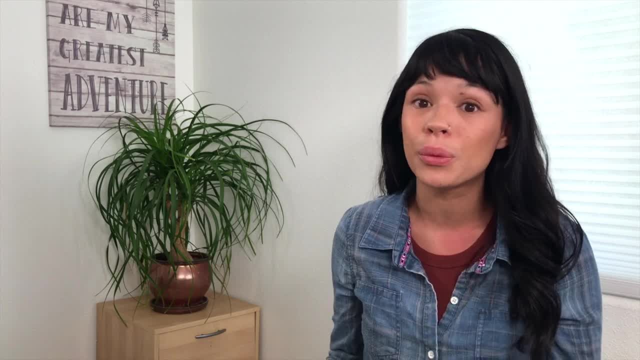 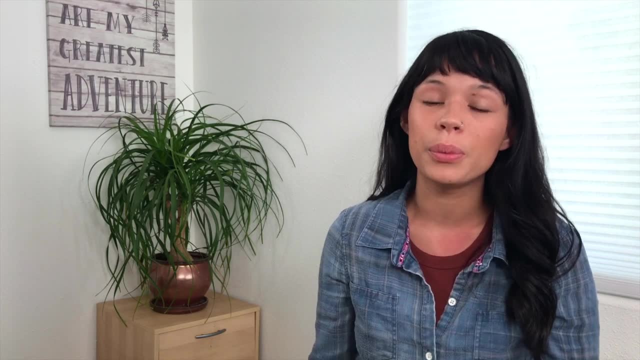 on its own. That's work that you, as the homeschool parent, don't even really need to facilitate. Focusing on reading really good quality books, otherwise known as living books, will really help with teaching all of these concepts, because these are books that have. 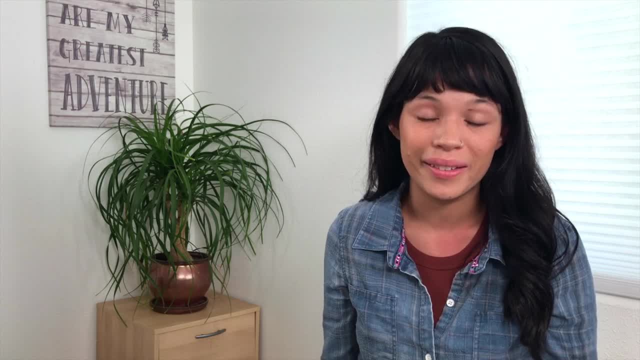 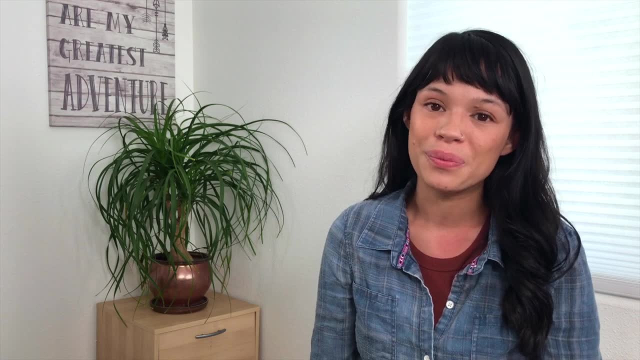 stood the test of time and also are just really high quality and well written. So that's something you need to keep in mind. to simplify language arts is to let the books do some of the work for you. Another tip I have is to combine handwriting skills with other language art skills. I know 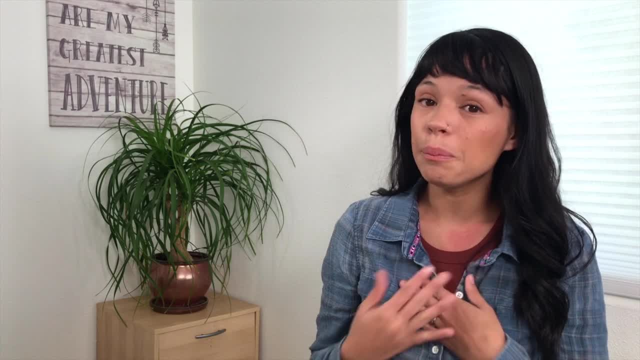 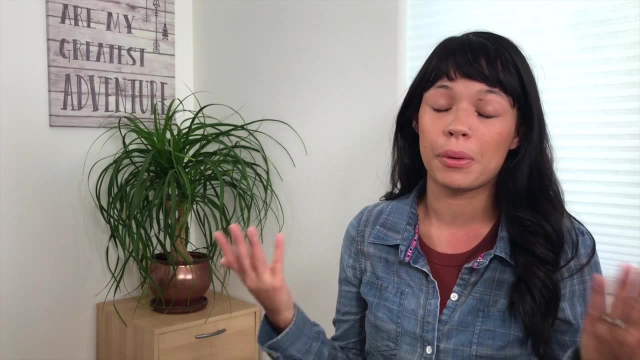 some people are kind of concerned with how their children's handwriting looks. I'm personally not really concerned about this. Maybe it's just because my kids have okay handwriting already, or maybe it's just my personality. But I think that if you are concerned with handwriting, 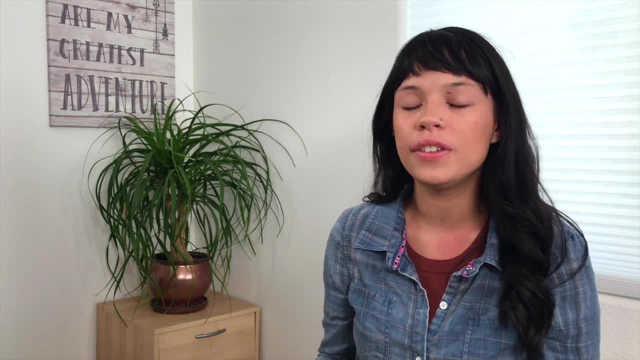 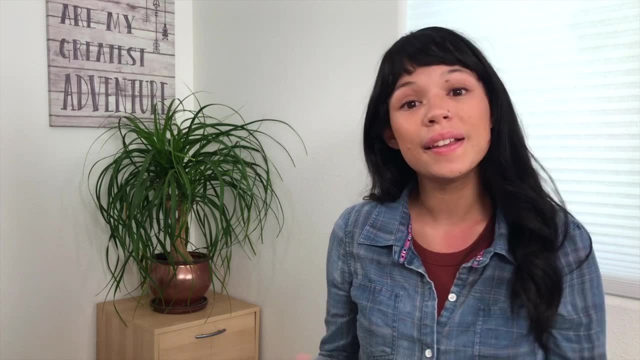 you can kind of lump this in with skills. What I'm trying to say is you don't necessarily need to invest time and money into a curriculum that is just for handwriting. An example from my own home school is we have always used Explode the Code and Beyond the Code. 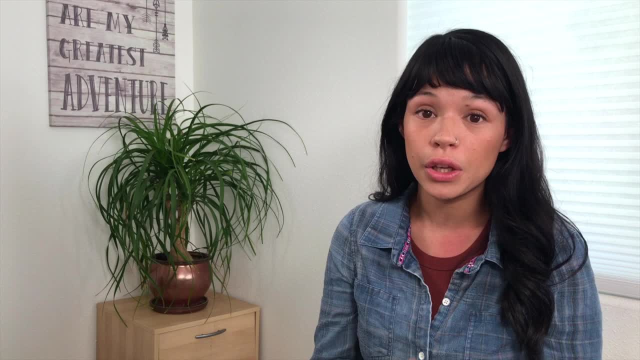 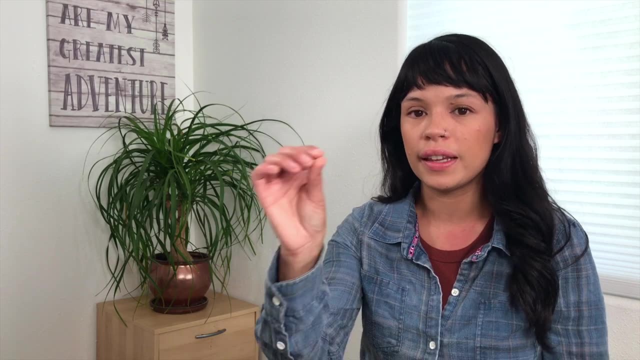 from the beginning and I know that the early Explode the Code books do help with handwriting a bit so that your kids are getting some practice in with like the dotted lines and everything to be able to write letters correctly and these are the letters that they're gonna be focused on it within the 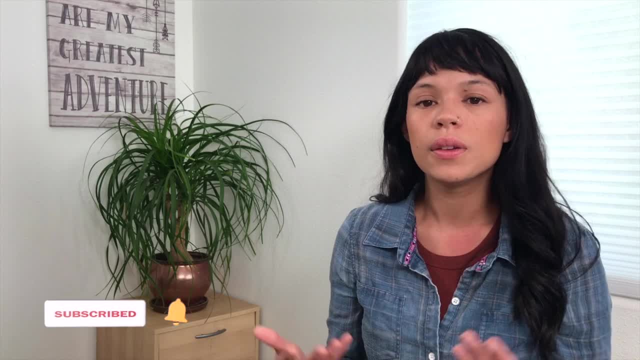 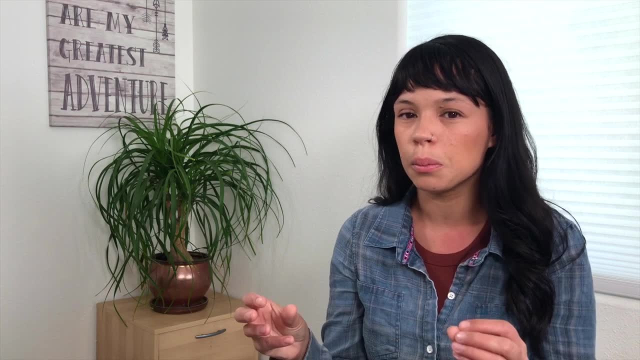 chapter and then you move on and there's lots of writing practice. so that's a good example of, you know, mixing phonics with handwriting, so you're not having to do two curriculums, you can just use one. Now an example that would kind of 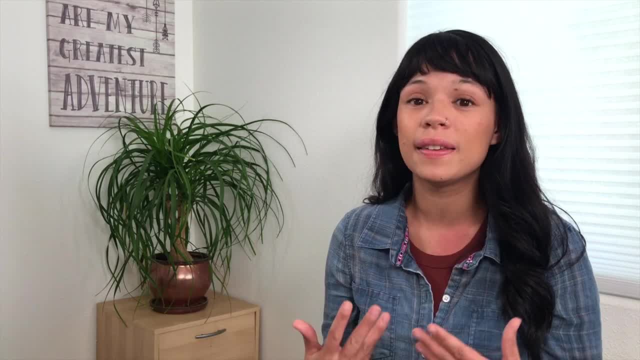 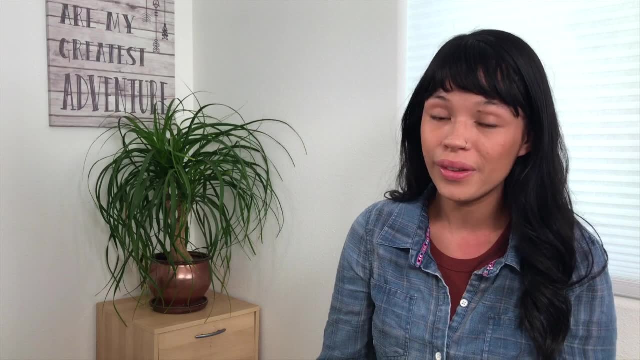 compartmentalize your home school a bit too much, in my opinion, is something like All About Reading. Now, I have nothing personally against the All About Reading curriculum. I have used it. it actually did work pretty well for my kids. but the only thing that I I don't know if you've heard of it, but I think it's pretty cool and I think it's 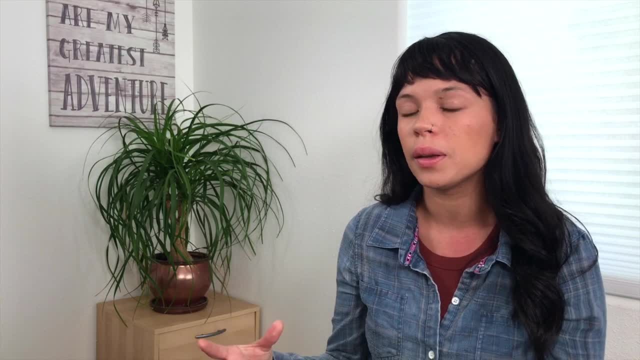 I don't know if you've heard of it, but I think it's pretty cool and I think it's didn't like. about it is that it didn't feel like a complete language arts curriculum because it is just focusing on the phonics and the reading skills. so 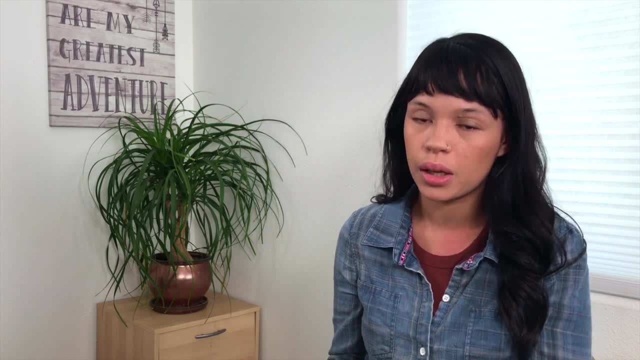 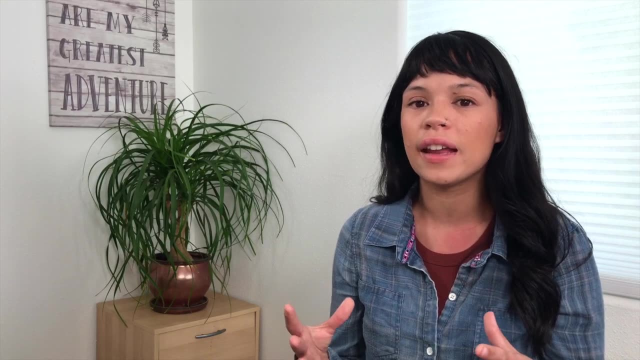 there is no handwriting practice, not even in the activity book. so that's one thing to consider when choosing any of these language arts curriculums- is how can it kind of be multi-purpose and serve multiple uses to you potentially, if handwriting or other things are ones you want to lump together? Another tip: I 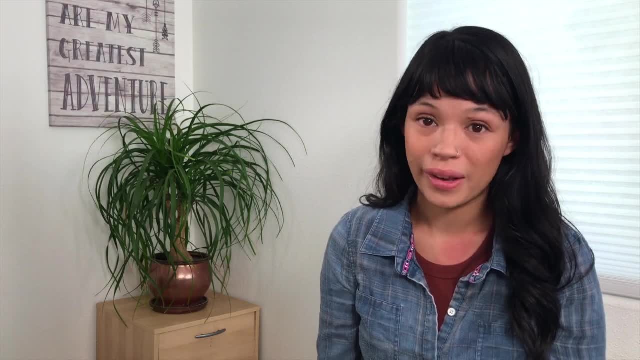 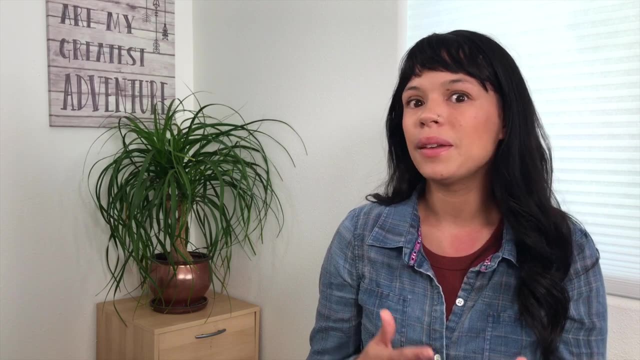 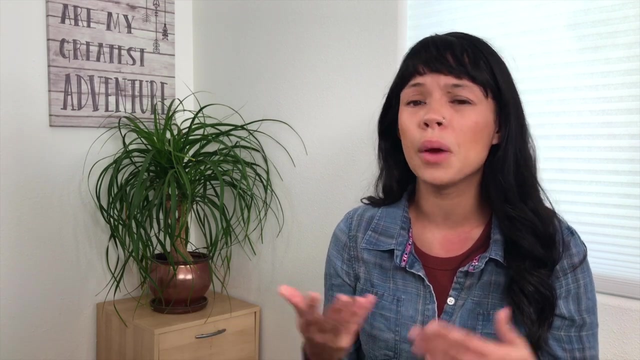 have is: don't stress about progress too much. I know it's easy- and especially with something like language arts, which is really measurable, to maybe fall into that pitfall of comparing your kids to other kids. Oh, my kid isn't reading yet, but that kid is. or my kid cannot write in lowercase letters yet, but 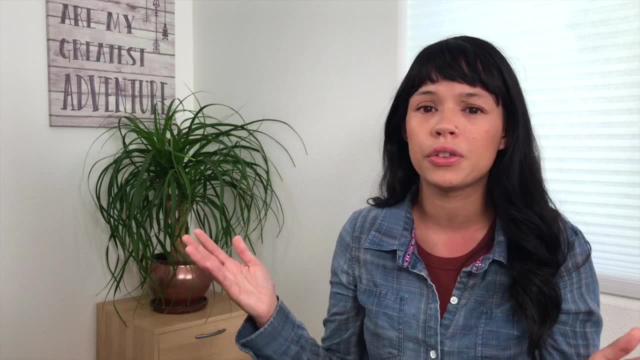 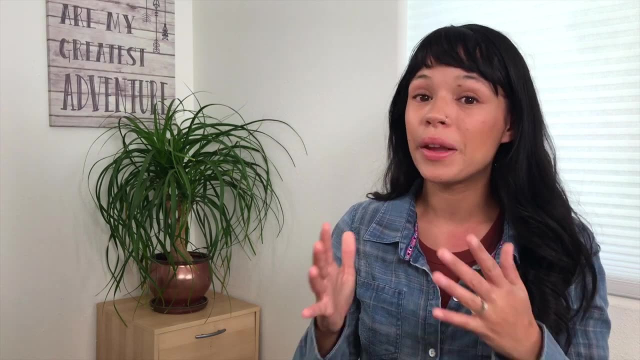 that kid is writing entire paragraphs with indentations and correct punctuation, Like it's so easy to fall into that pitfall. but you really can't do that with something like language arts. I can promise you from my own personal experience that these skills sometimes just come in time like 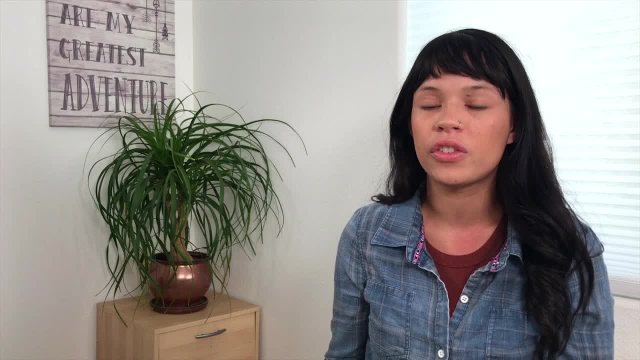 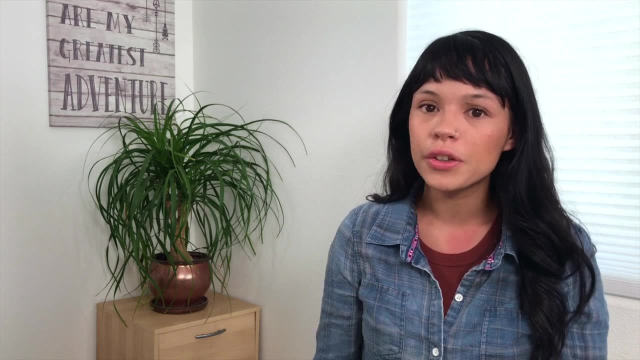 overnight your kid might just develop a little bit of a skill and then you're gonna develop a love for reading or just even just the. the ability to read sometimes comes kind of overnight. So just stick with what you're doing, be consistent, and that progress will come in time. I don't want you to worry about. 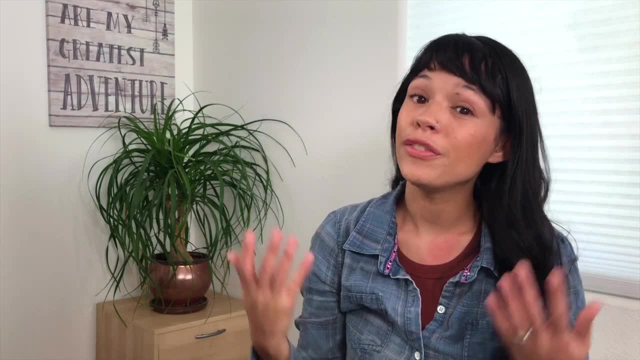 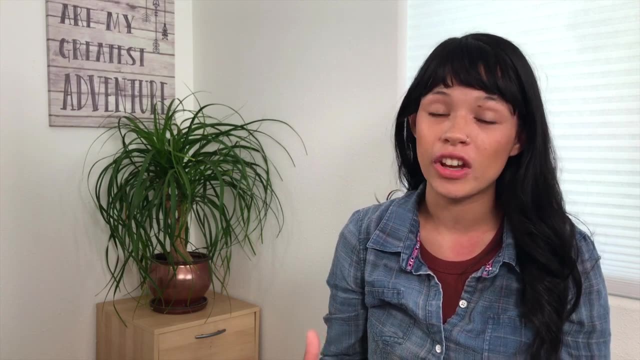 falling behind or feeling like your kids are late to the game. If you do feel like you do have some legitimate concerns about your child's progress, there are ways that you can get extra help. in just this one area of language arts You can maybe try a super specific curriculum to the specific need you think needs to be. 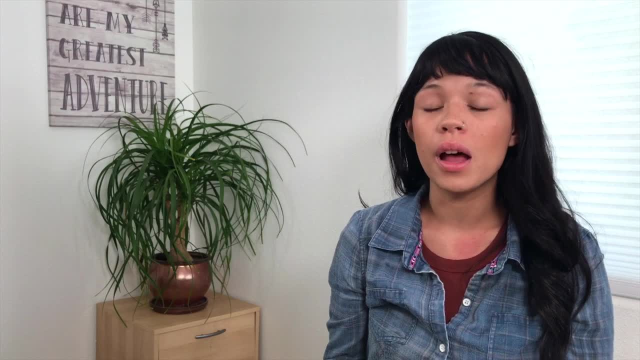 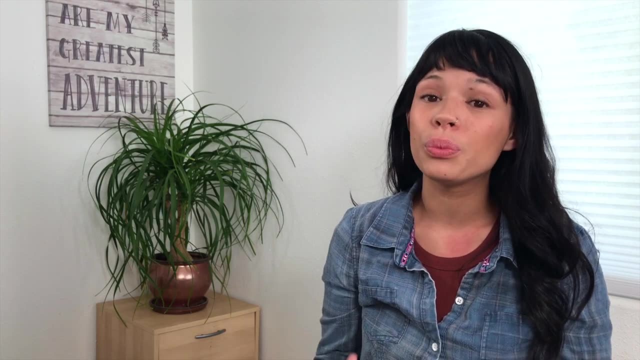 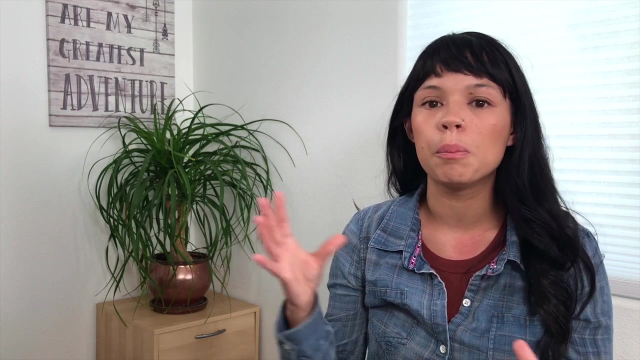 taught. You can get tutoring. Some vendors for homeschool do offer classes in certain concepts of language arts. So if you do really feel like there is something that your child is just not getting, no matter what you've tried, try thinking outside the box. Maybe you know, pull in one of these extra resources and 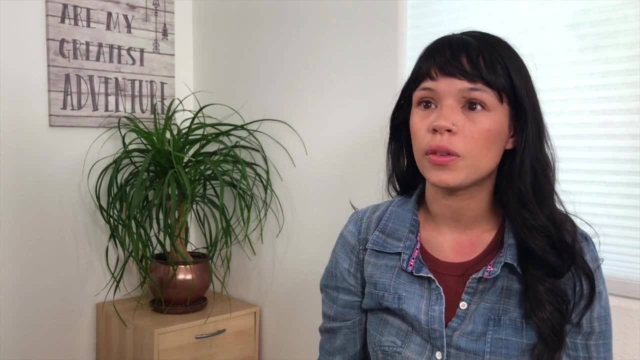 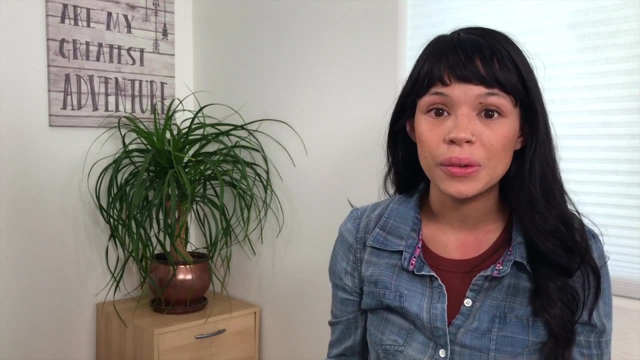 see if that helps. For example, for me. my oldest daughter just was not wanting to read and she was way behind other kids I saw at her age She didn't even have the time to read. So what I did is I started this thing called Free Reading Fridays. I 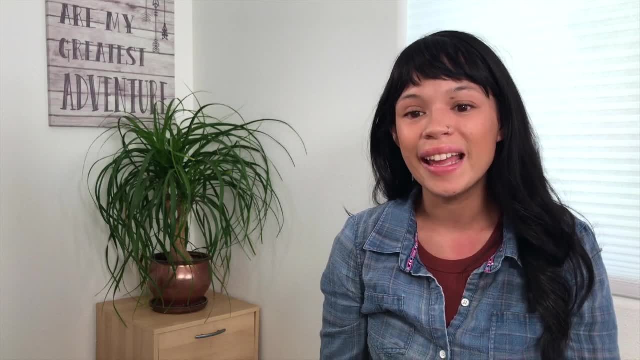 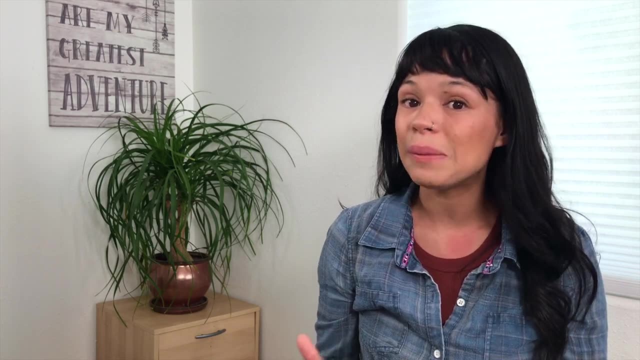 did a video about it so I'll make sure to link to it for you. and we just made that time just to independently read and make reading fun, not a chore. It really made all of the difference for her. It gave her that space to just read for. 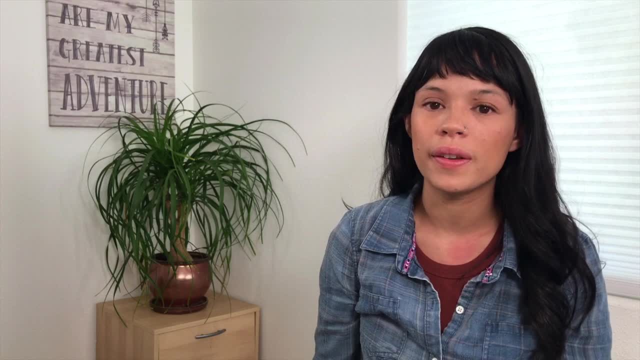 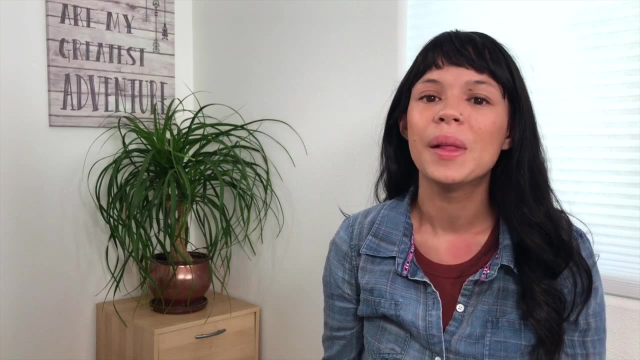 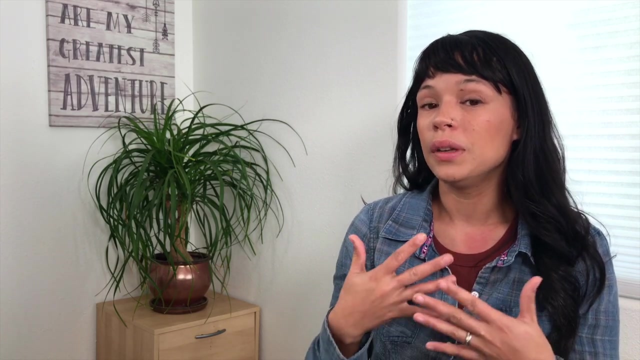 pleasure's sake. I guess the main point with not stressing about their progress is that the stress is going to be felt by your kids and then it won't feel fun anymore to read or write. So I just want you to make it as fun as possible and as accessible, and don't bring your own feelings about you. 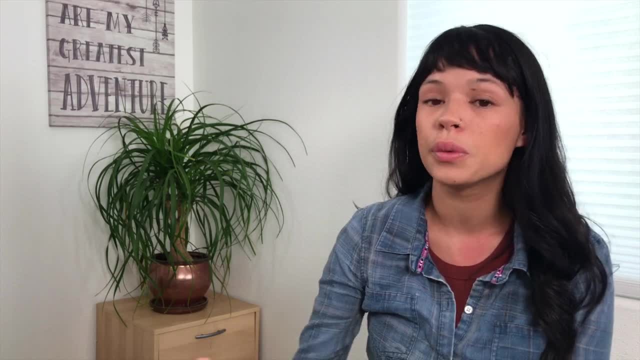 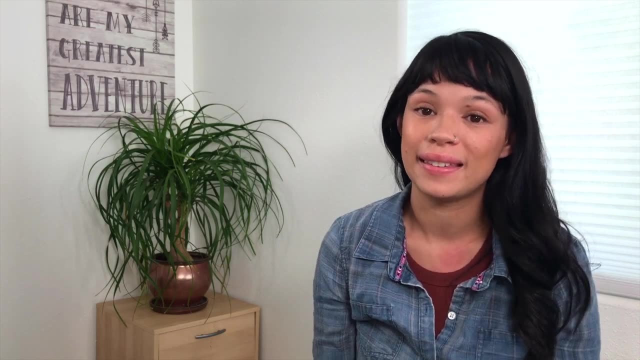 know. oh, I'm scared that my child isn't progressing into your home school because that's not gonna benefit anyone. So, in closing, if you had to take just one thing away from this video, it is this: As long as you continue doing read alouds or having your children read, I think that all other language arts 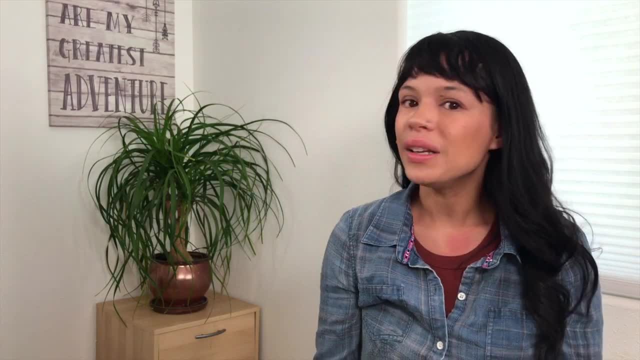 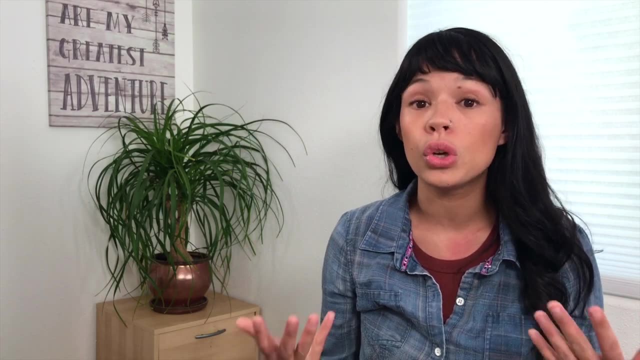 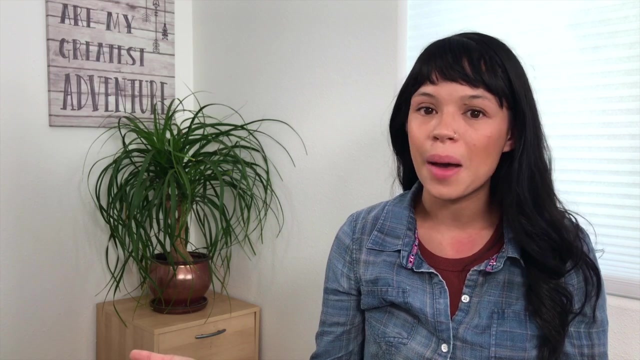 concepts will be learned by them in time. You don't need to rely on expensive curriculum or follow the standards to achieve your goals. You don't need to rely on money or authority. Just have them exposed to good quality books and have them read on their own. Read for fun, and everything else will come naturally. 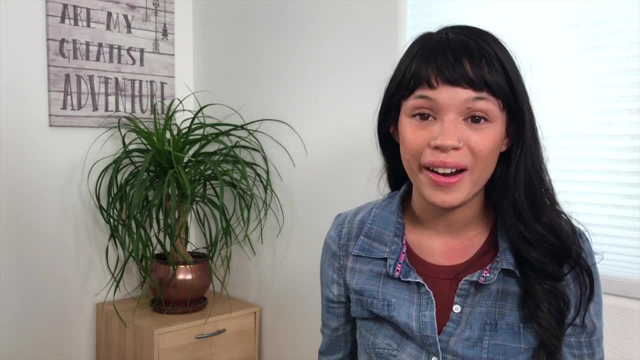 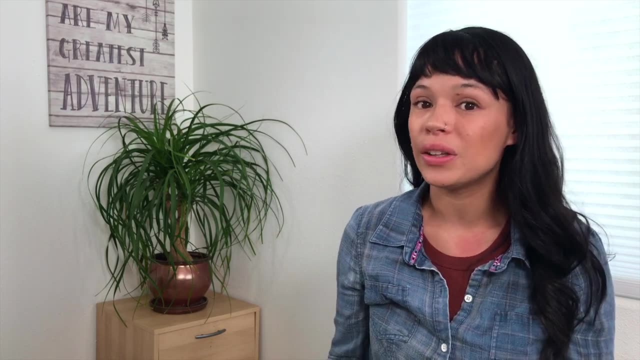 I mentioned it before but I'll mention it again: I did do a whole video on free reading Fridays, so I will make sure to link to that over here so you can check that out. next- And I know I mentioned Explode the Code because I think it's a- 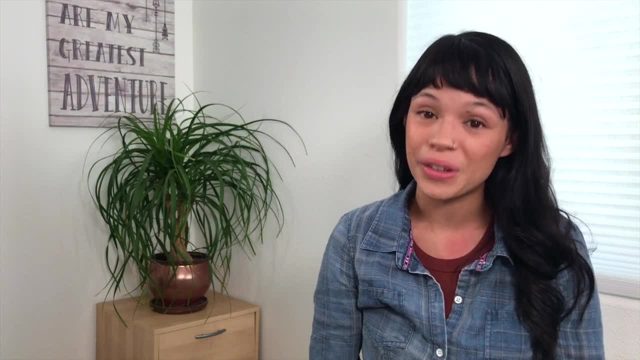 great use of handwriting practice and just phonics. so I will also put a link to my review of Explode the Code over here so you can check it out. See you next time. Happy homeschooling. 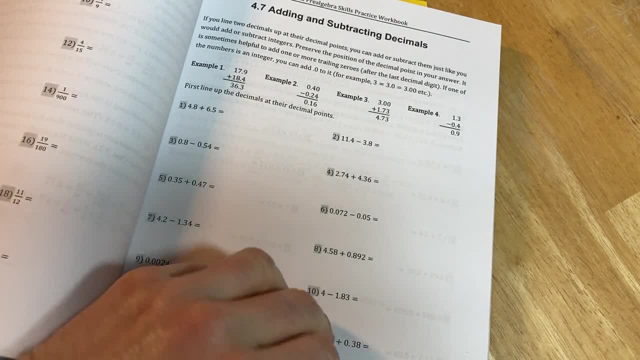 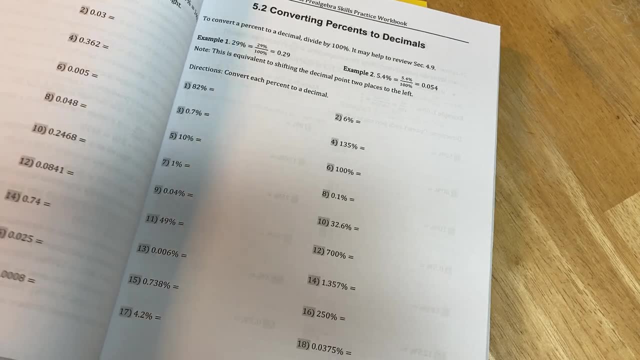 What do I mean by a super beginner? I mean someone who just doesn't know much mathematics. You know, if you have been out of school for a while, or you just didn't do well in school, or maybe you're just learning it for the first time because you've never seen it. If for 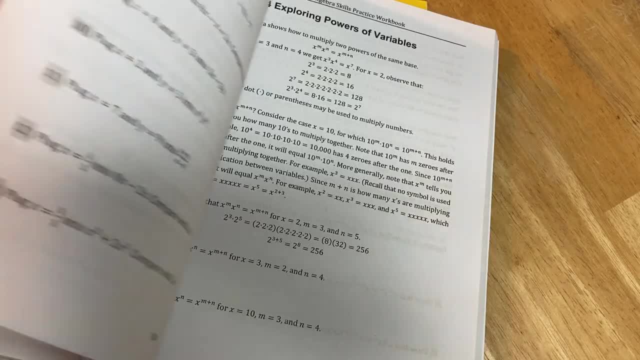 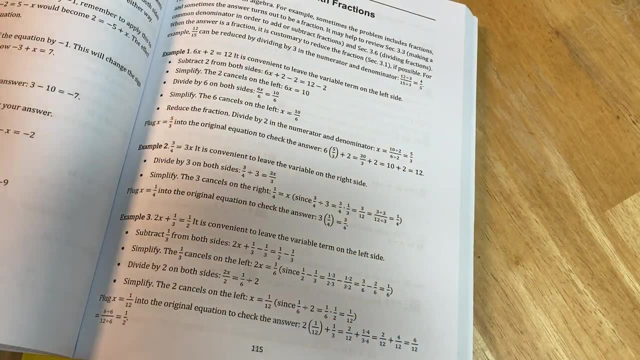 whatever reason you feel like your math is really weak, then in this video I want to show you how you can change that, and I'm going to give you two options: One is for like super, super beginners and one is just for like super beginners. So let's start with. 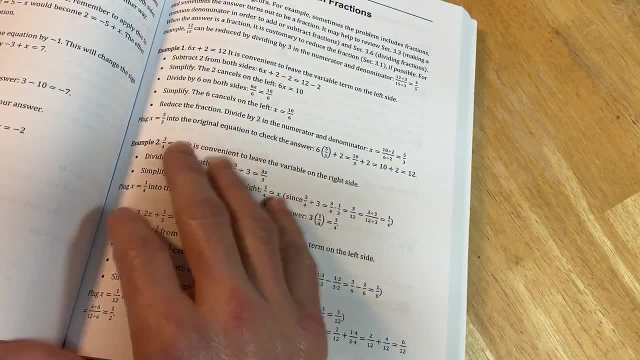 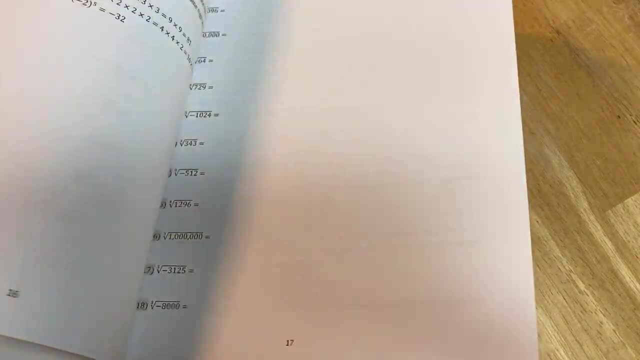 the one for super, super beginners. So if you feel like your math is really, really weak, so like you just barely know how to add and subtract and stuff like that, then you want to look at something like this: This is an option. Now, this is not a textbook. 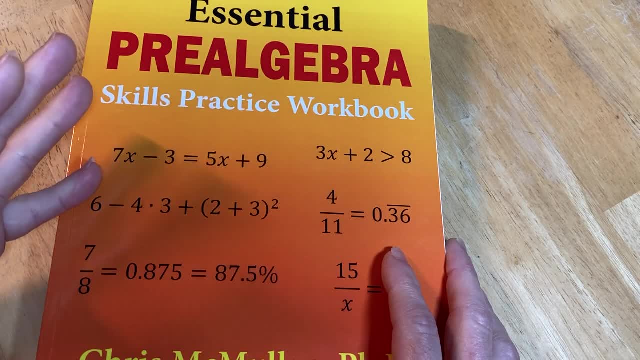 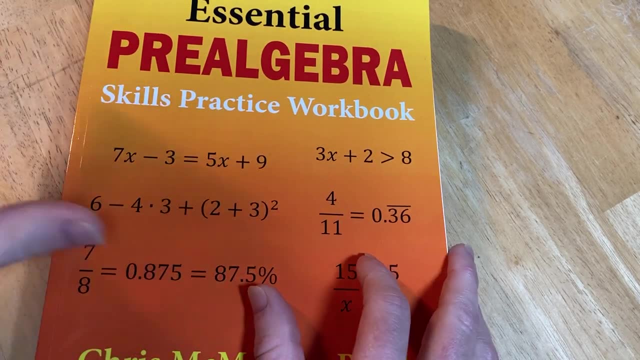 This is a workbook, which means that it has answers to every single problem and you can actually write in the book. It also means that it's super inexpensive. That's another reason I wanted to show you this one. It's called Essential Pre-Algebra.